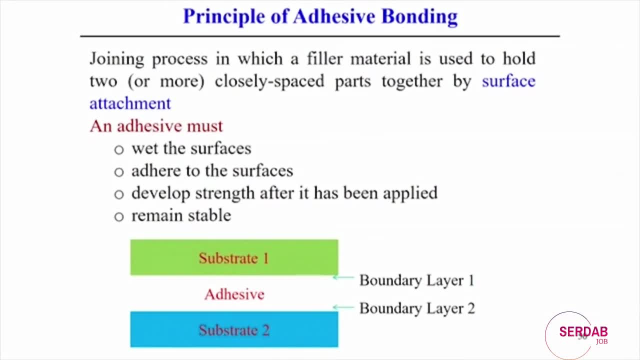 type of the filler metals, or filler metals means here the adhesives, with or without the application of the heat may or may not be the necessary of the application of the heat, So the in that way this is different, Thank you, from the any kind of fusion, welding processes or bridging and soldering process. 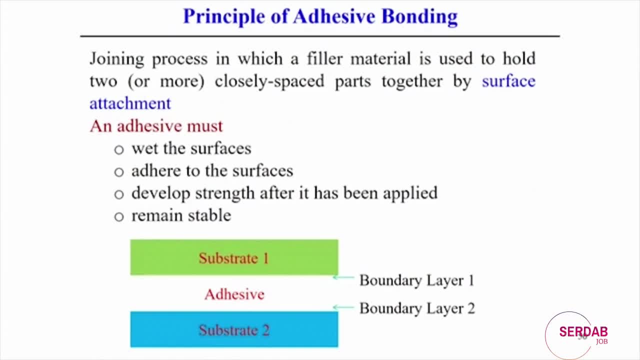 So when you use the adhesive to join between the two substrate, if you look into the figure, in this case the substrate 1 and substrate 2 will try to join using some adhesive. So the most important factor using the adhesive, the type of the adhesive. second important: 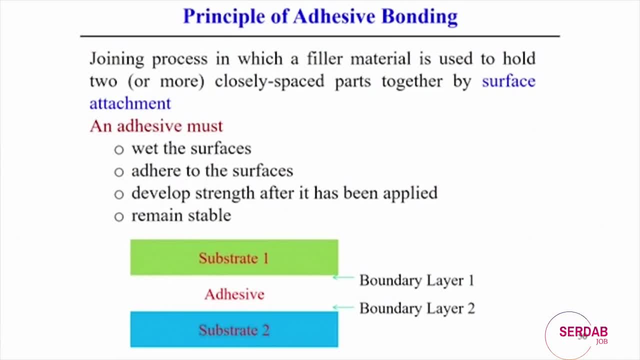 point is that when you join substrate 1 and substrate 2, what will be the gap? that means, what will be the thickness of the adhesive? the joint strength of the joint can vary depending upon the nature of the adhesives and depending upon the thickness of the adhesives. 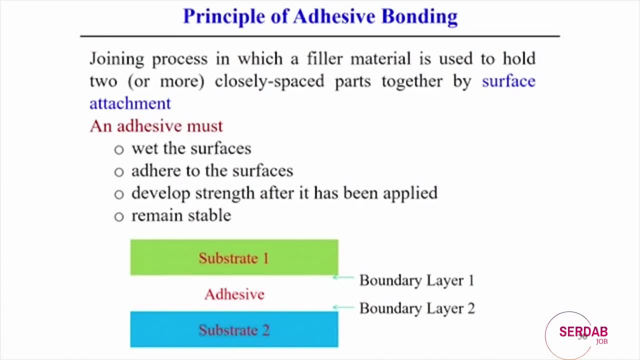 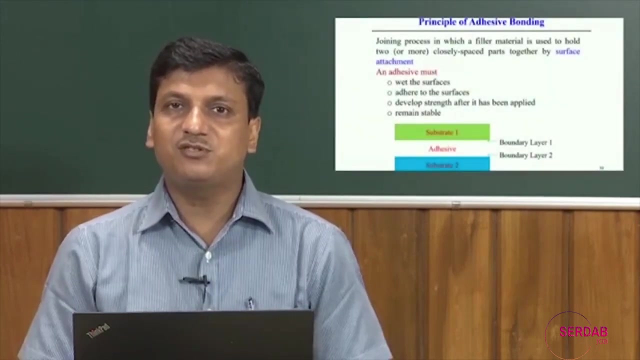 And may be other secondary requirement are also there to get a successful weld joint simply by adhesive bonding. So in principle, that it follow the surface attachment Between the two components. So therefore, when you use adhesive should have some quality such that it will try to wet the surfaces, both the surfaces, when, which surfaces we are? 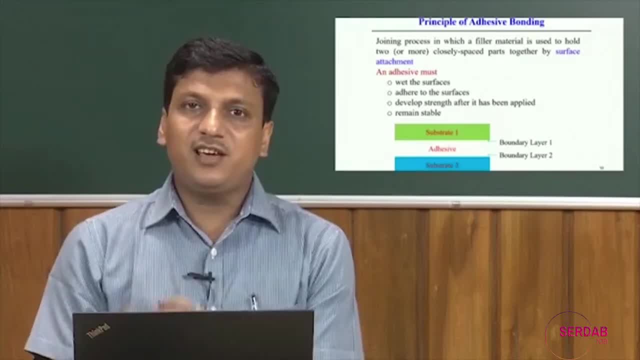 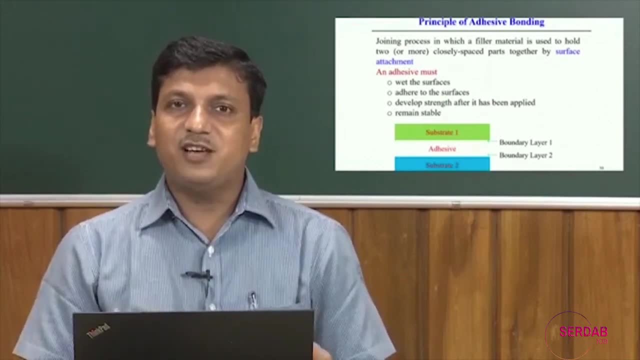 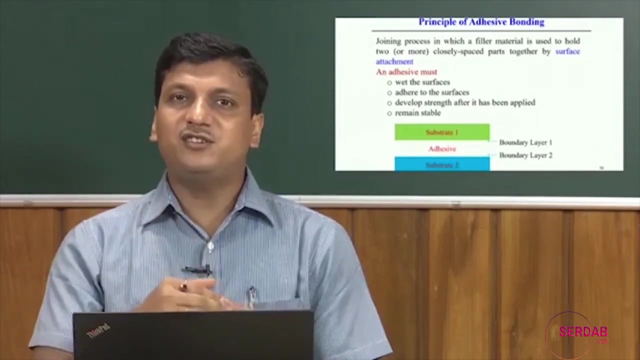 supposed to join And it exactly adhere to the surfaces and develop the strength after it has been applied. that means when sometimes the simply putting the adhesives- and there is a necessary to keep it- keep hold on for a long time, And then that is called the. 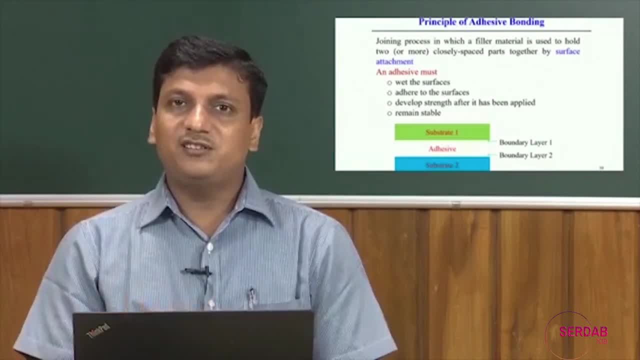 curing process. so in that after curing they the joint between this two surfaces and simply wetting the surface and but this joints should be remain stable a certain period of time. And there is a element point which goldenreiben is these adhesives. it may not be 100 percent. 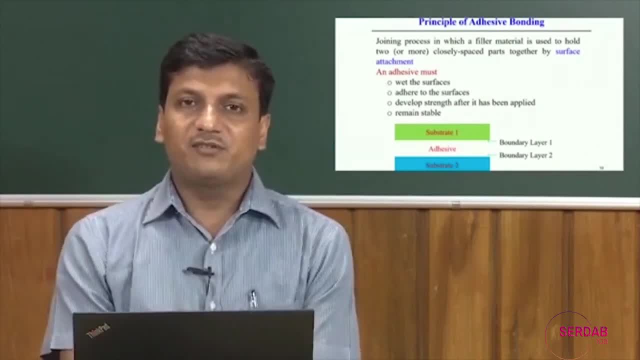 stable for 20, 50 percent. So the point is, if you told the adhesives are knew one, the adhesives theADDESSIVEPRODUCTION general, So this adhesives one glimpse size. ok Then, so the you do to uploading. So this adhesives one After the adhesive bolt with the other You mainly are know. so there is a necessary to keep it, keep, keep, hold on for a long time, And that means that is called the curing process. So in that after curing the, the joint between 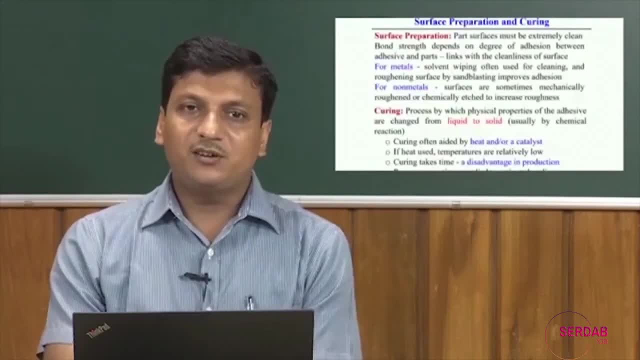 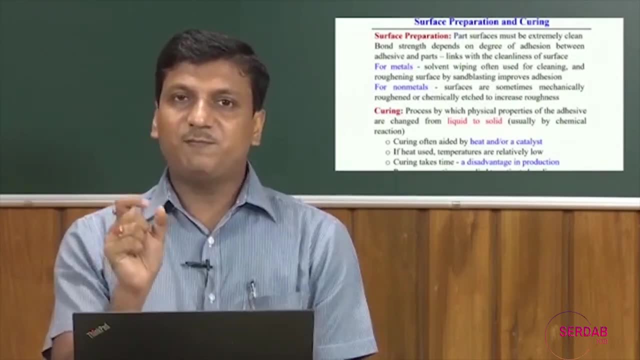 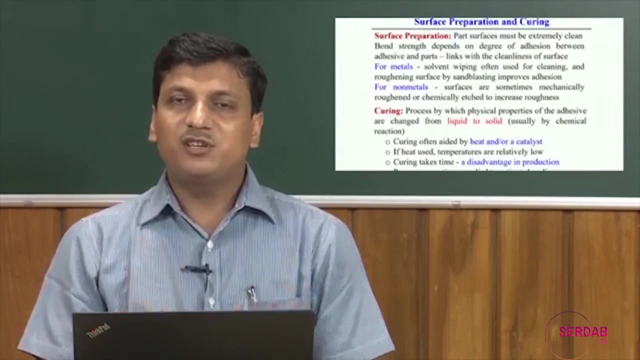 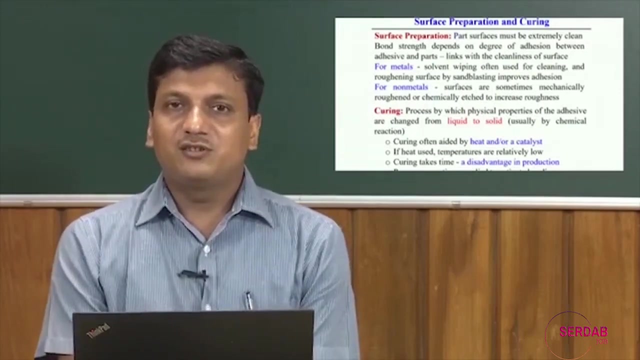 successful joint using the adhesive bonding. there may be some that this process can be explained in the two terms. One is the surface preparation and the curing. These are the two significant terms. based on that, adhesive bonding can be explained in better way. First, is that surface preparation, So definitely the work piece? surface like fusion. 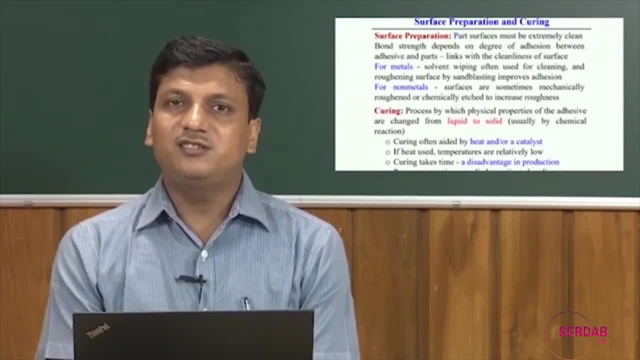 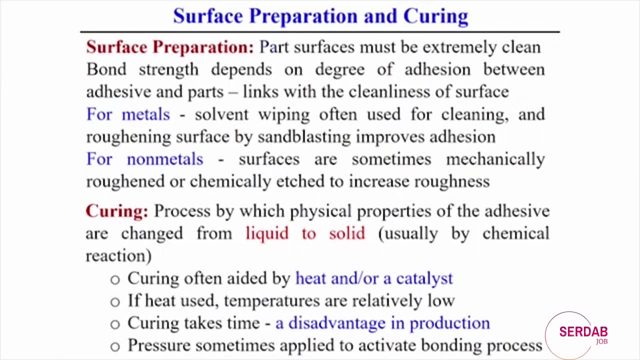 welding process. also, to get the successful weld joint it is necessary to the clean the surfaces of the work piece or substrate material before welding. Similarly, here also some surface preparation are necessary to get a successful weld joint by with the application of the adhesives. So part surfaces must be extremely clean such that because the bond 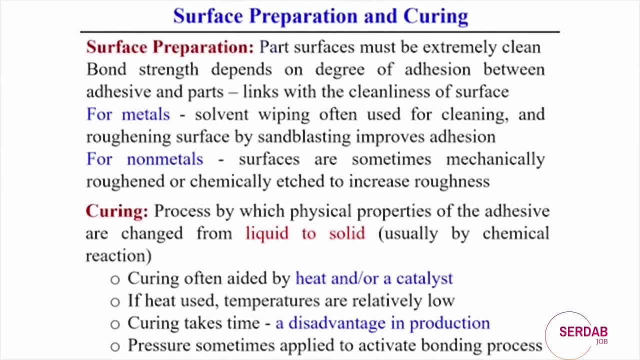 strength Depends on the degree of adhesion between the two surfaces or two adhesives, between the addition between the surface and the adhesives and adhesives and the parts That actually very much links to the cleanliness of the surface. So therefore extremely clean. 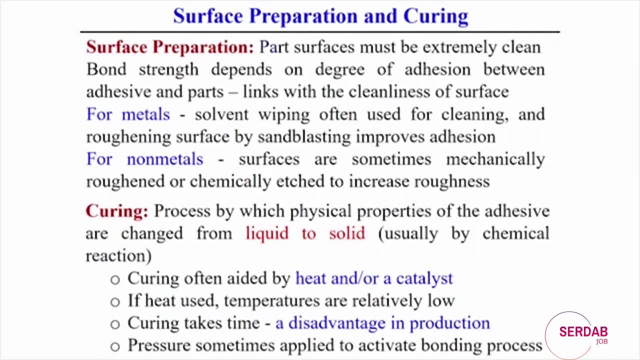 surface is required in this case. Second, but other points for the surface preparation. this I mean, I mean how we, how the surface preparation can be done in case of the metals and in case of the nonmetals. So in case of metals they actually we using the solvent wiping after. 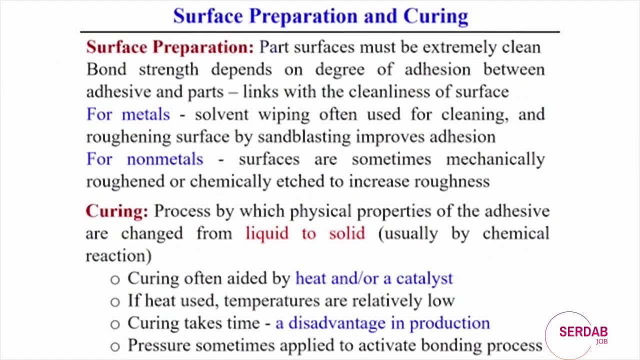 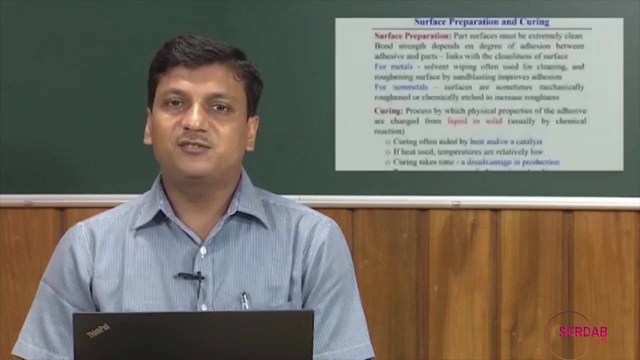 use after use for the cleaning. often use for the cleaning purposes and then roughening of the surface is also required. Sometimes the sandblasting techniques is required to improve the surface roughness of this material. but surface may not be too rough. then there may be the other difficulties, but certain roughness is required So that wetting action. 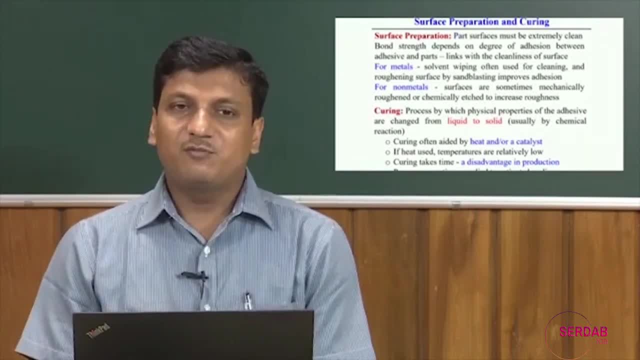 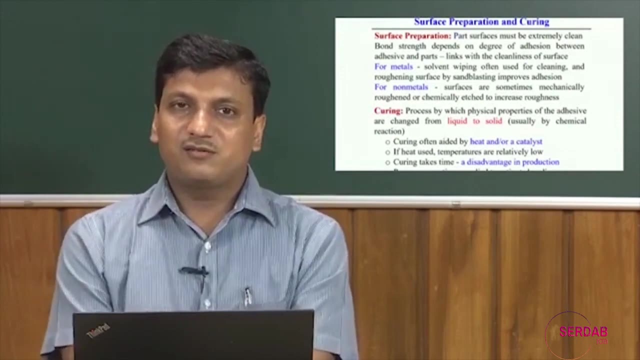 can be good by the adhesive to the surface. but for nonmetals the roughness is improved, sometimes the mechanically, or sometimes we can use the chemical etchant also to increase the roughness. In general the surface preparation for the adhesive bonding is the first one. the cleanliness. 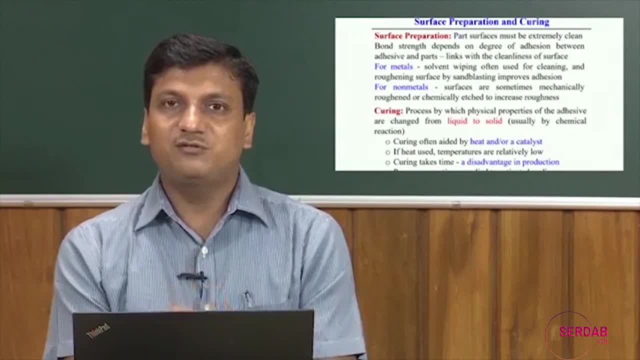 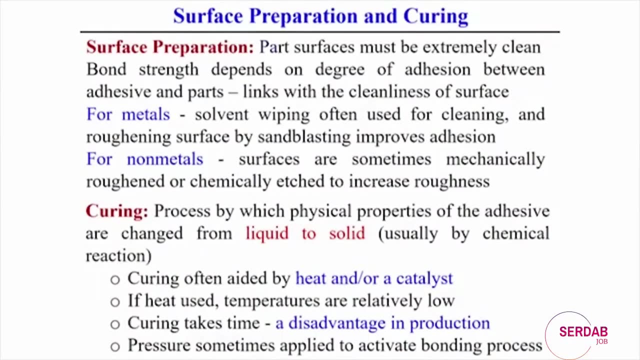 second secondary thing is that some sort of roughness should present in the surface and next curing. there is another component of the adhesive bonding is that curing action? So this is the process by which the physical properties of the liquid adhesives changed. when it is changed to the solid, comes to the solid phase. 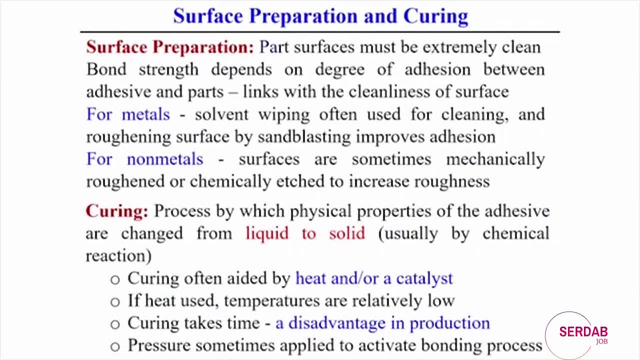 So that comes usually some by some chemical reaction. So in this case the curing can be done carefully in the adhesive bonding process. So it is open, used by the by curing can be done with the aid of the heat sometimes, or sometimes we can use the some catalyst for. 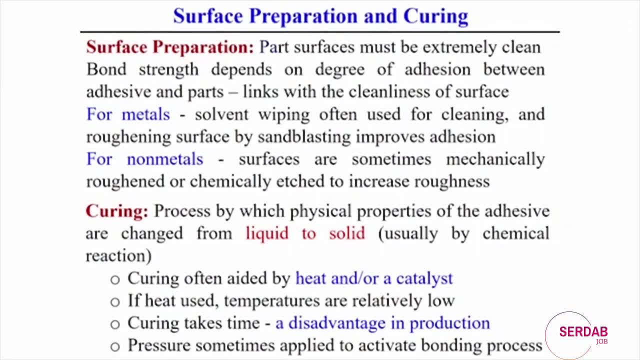 the curing purpose of the adhesives. So if there is a need of the application, application of the temperature during the curing purpose, but that temperature may not. 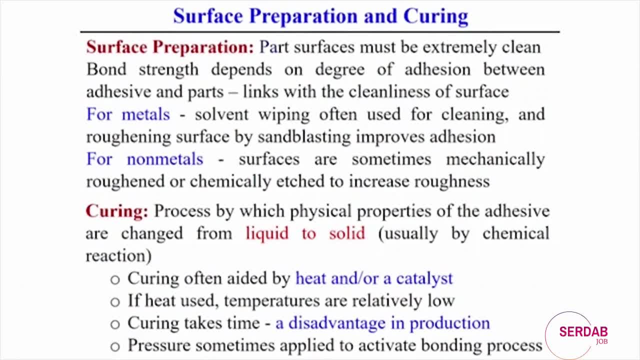 be too high. it should be very low, relatively low. But the main disadvantage of this process is that curing times is relatively takes a very long time. So that is why production rate is relatively slow in this case. So that is the disadvantage of this process. So sometimes it requires to applying the 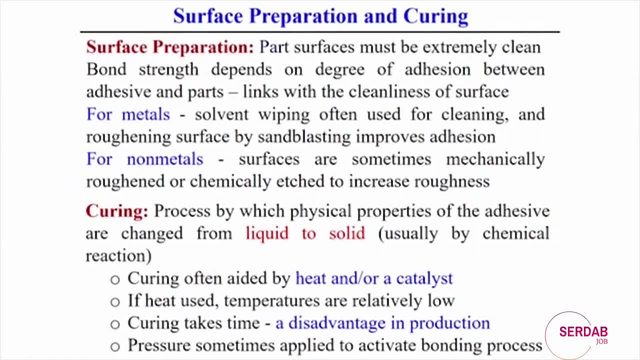 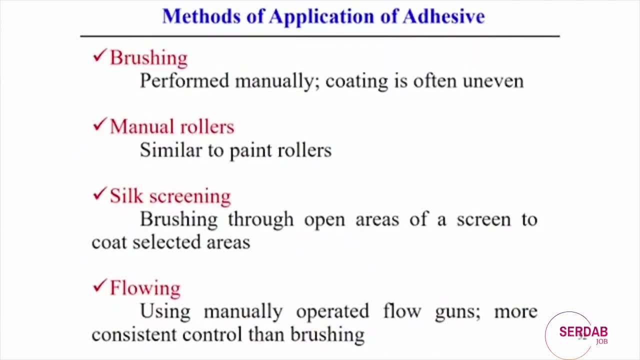 pressure also, So that applied pressure activate the bonding between the two substrate materials. So what? now we come to that point that what are the typical methods of application of the adhesive, What way we can put the adhesive between the substrate material? So simply, 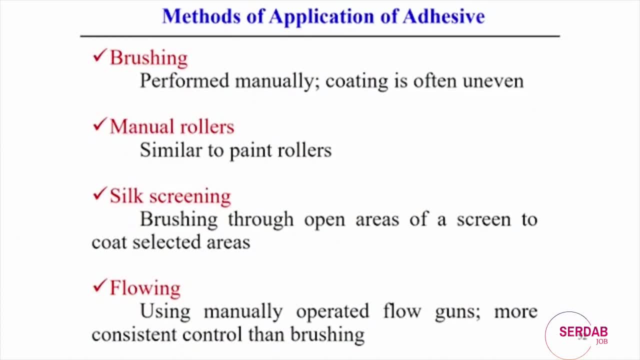 manually we can do the simply brushing. but when you do the manually, this thing, there is a possibility of the uneven coating may not be the coating may not be the very even And that means there is a variation of the thickness over the surface. So that is the one thing, the simply brushing. 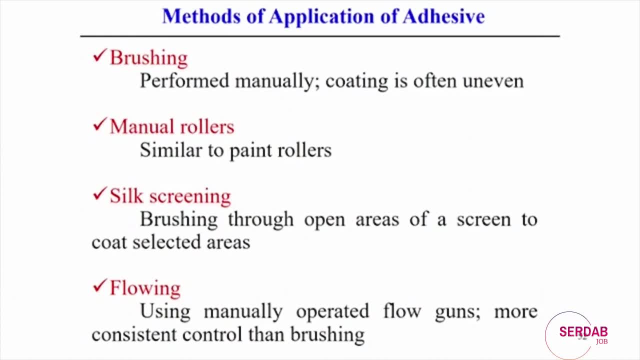 Sometimes we can use the manual roller, similar to the paint roller, but in this case definitely we can maintain the smoothness of the surface And but since it is doing the manually, so there may be the possibility of the variation of the thickness also. 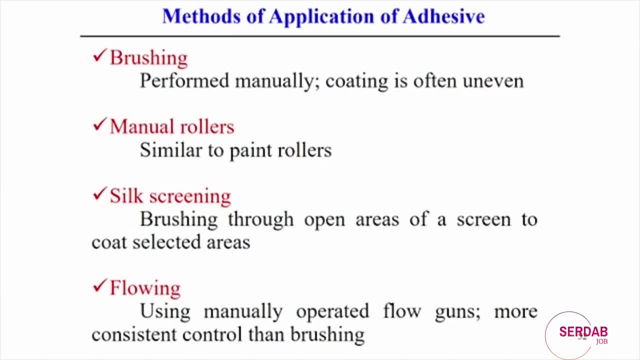 Silk screening also. sometimes this is the another methodology to application of the adhesives, So simply brushing through the open area of a screen that actually used to coat the selected. If you use the screen, it is possible to use the putting the coat. 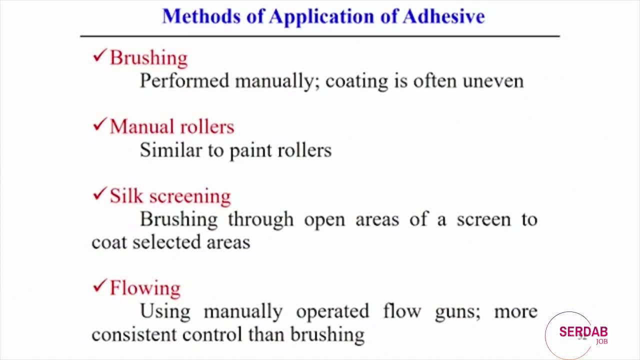 of the selective part, selective area or selective area of the component. So this method is sometimes applicable to application of the adhesives and flowing. So usually sometimes you use the manually operated gun. from there you can see the motion of the adhesive. So 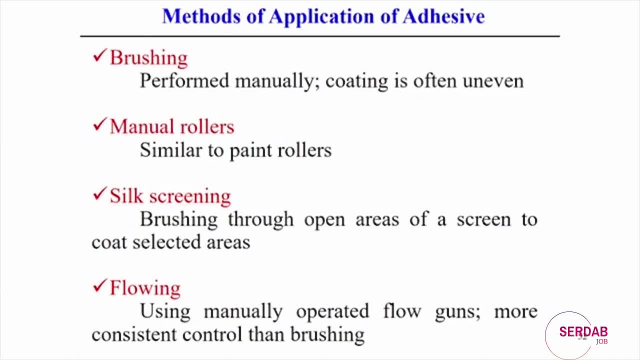 gun, for flow gun. basically that is required and when there is a consistent control of the consistent control is required and advantageous as compared to the simple manual brushing process. So this typically typical methods for the application of the adhesives to the substrate material. So after application of the substrate material then there is a 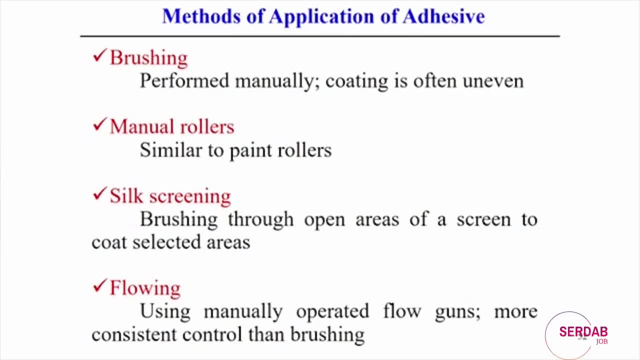 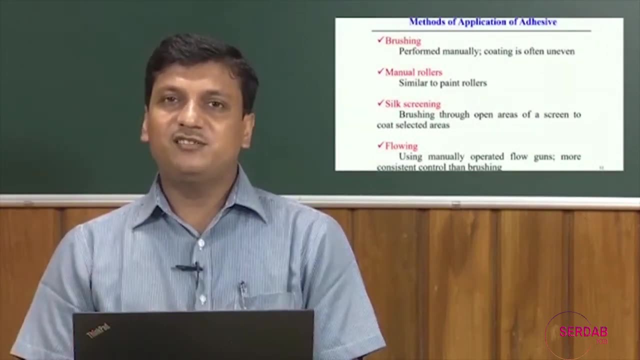 need, may or may not need, of the pressure aid of temperature, or sometimes we can use the, these adhesives, we along with some catalystic element so that it can accelerate the chemical reaction during the process, So that it can the curing can be done. 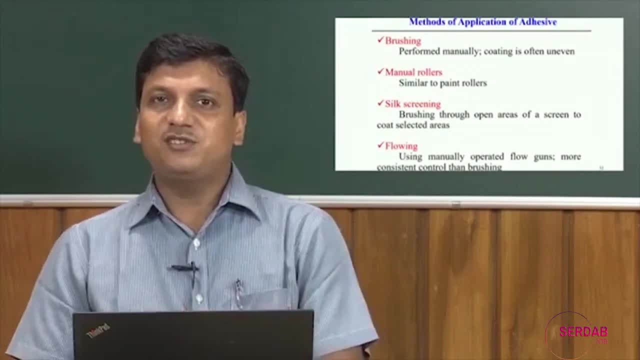 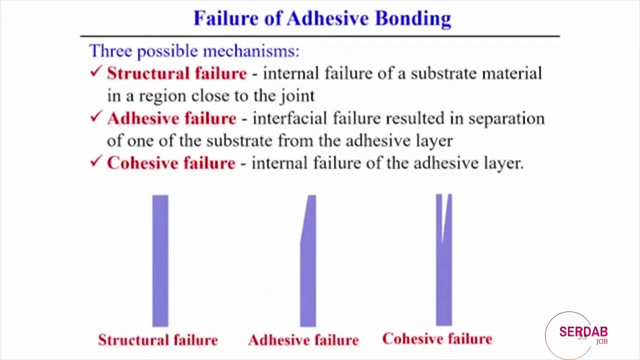 be done. That means the change of phase from liquid to the solid phase can be done quickly. also. Now, if you look into the typical failure modes on the adhesive bonding, when you, after the making the bonding, the, what are the typical failure mode of the adhesive bonding, the? 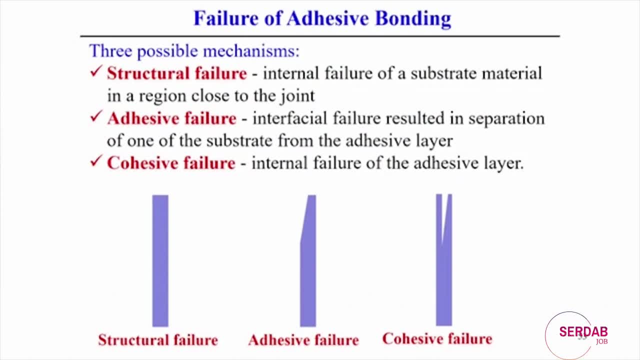 three possible mechanisms. One is the structural failure. here we can see the internal failure of a substrate material in the region close to the joint. So failure is more to the substrate material, with structural more to the substrate material, not actually the not. failure exactly happens inside the components of the adhesive adhesive part. 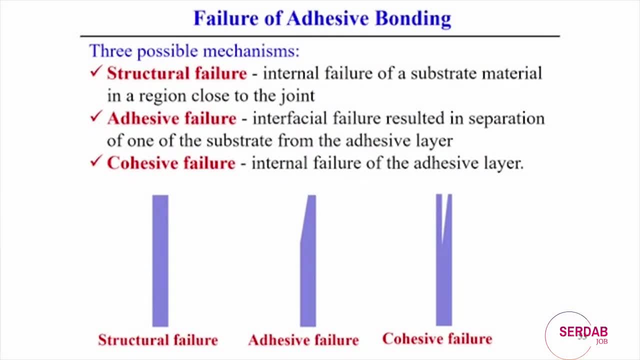 Then adhesive failure mean interfacial failure resulted in a specimen of one of the substrate from the adhesive layer So near about the adhesive layer there is a failure. if figure adhesive failure figure here, you can see there is a small component of the adhesive. 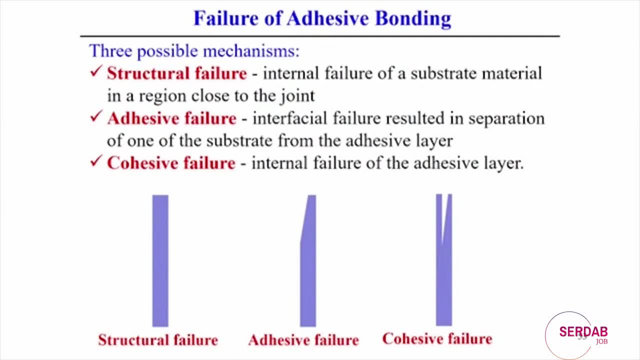 is disappear. So actually, fear happens near about the substrate material and one layer is absent in this case. So that is the typically called. the typical mode is the adhesive failure, Cohesive failure if the internal failure occurs in the adhesive layer. if you see, look. 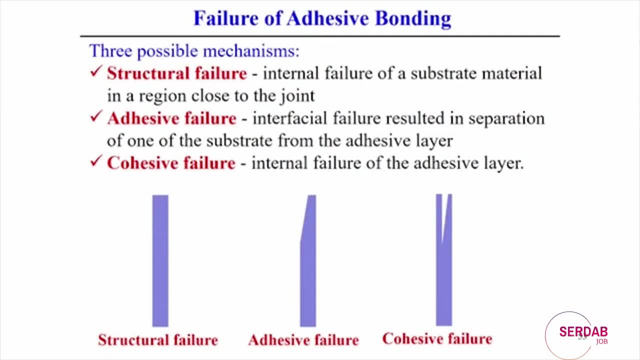 into that. seeing it is a completely failure is completely on the layer of the adhesive, within the adhesive volume itself. that is called the cohesive failure. So these are the three different types of adhesive failure modes we observed in case of the adhesive bonding. Now, classification of the adhesive. what are the different types? 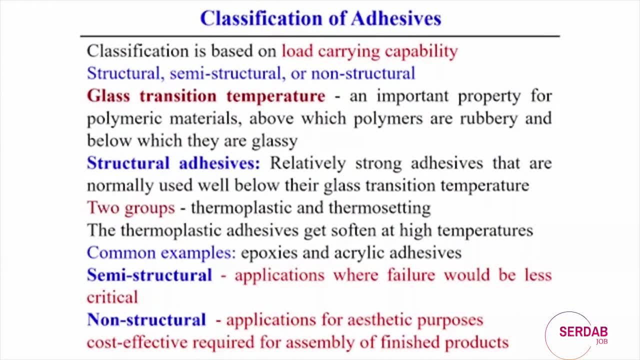 of the adhesives can be used that are different way, or different types of the adhesive materials be used for the adhesive bonding. but here we try to do the classification based on the load carrying capability. So, depending upon the load carrying capability, the adhesives- 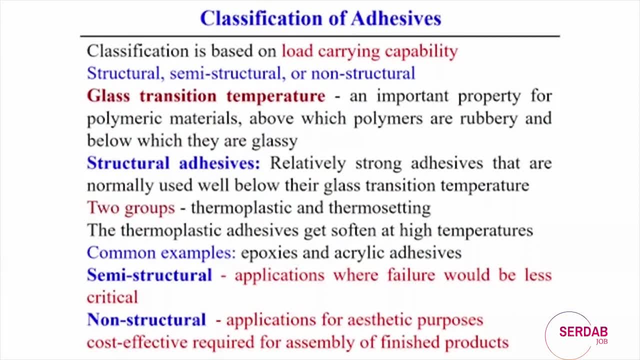 can be defined as the structural, semi structural and non structural. These three different types of the classification can be done based on the load carrying capability of the weld joint using the adhesives. But to do that one is the important point is that glass transition temperature, which 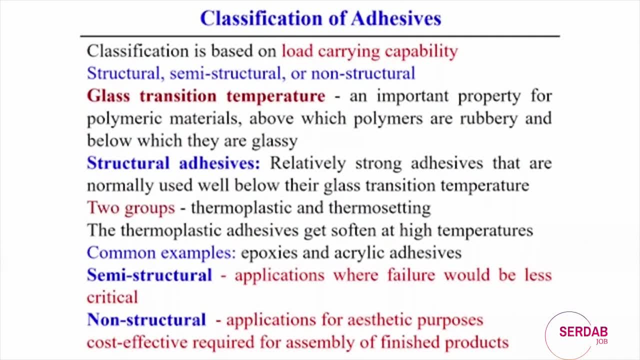 is very much related to the polymeric material and that the temperature decides in such a that above which the polymer are rubbery like polymer, becomes like chewing gum, Large deformation can be done, and below which it is like a, the glassy type of structure we 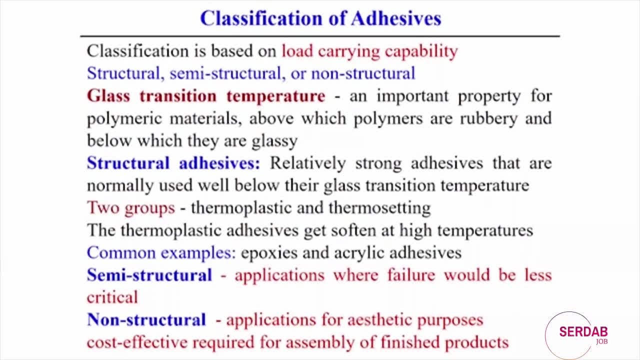 can observe, So that sometimes we use the, So that sometimes we use the, So that sometimes we use the polymeric material. or may be that the important temperature is the glass transition temperature, which is may be equivalent to the melting point temperature in case of any. 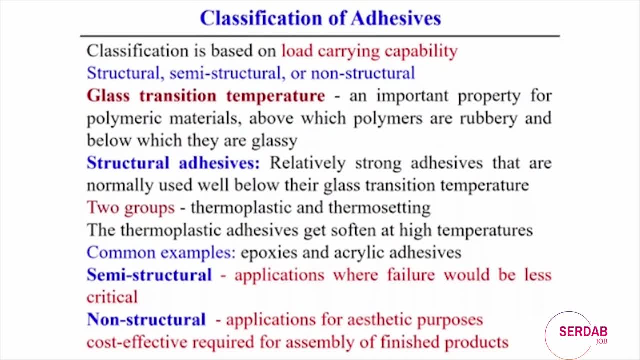 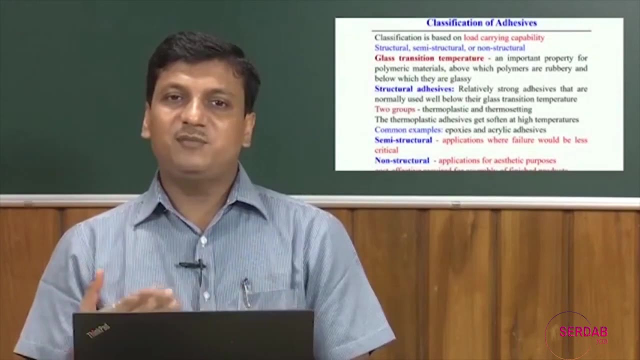 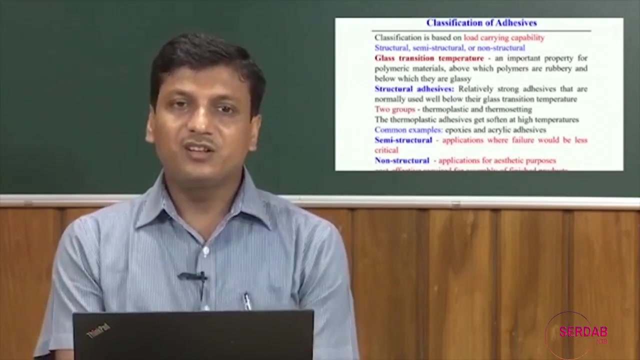 kind of metals, any kind of metals. So structural adhesives are basically the relatively strong adhesives that normally used, basically well below the, their glass transition temperature. So well below the glass transition temperature. that means the adhesives looks like here, the it is written, the structure like the glossy structure. So two groups: thermoplastic. 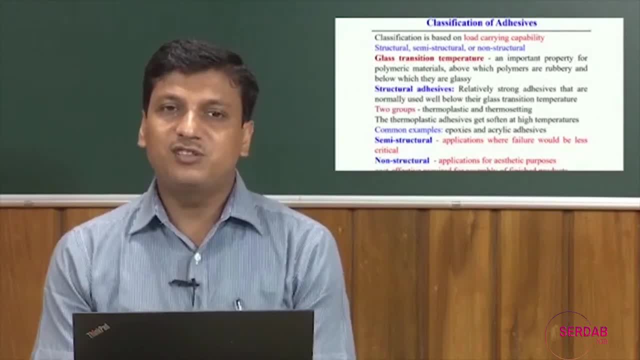 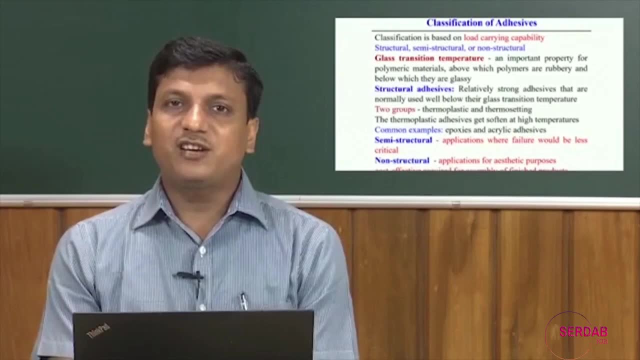 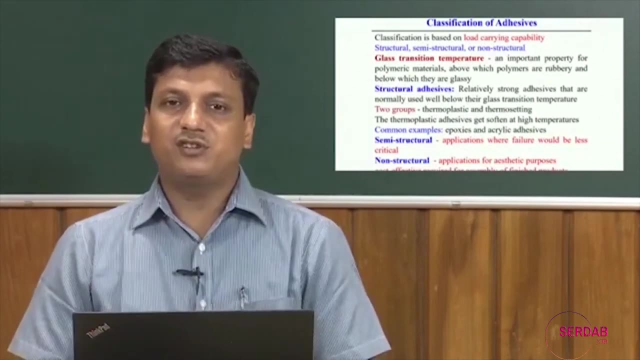 and thermosetting, thermosetting, thermoplastic groups they actually form. they can be examples for the structural adhesives, But we know that thermoplastic and the thermosetting plastics thermoplastic. they actually becomes open, softened at the basically high temperature. 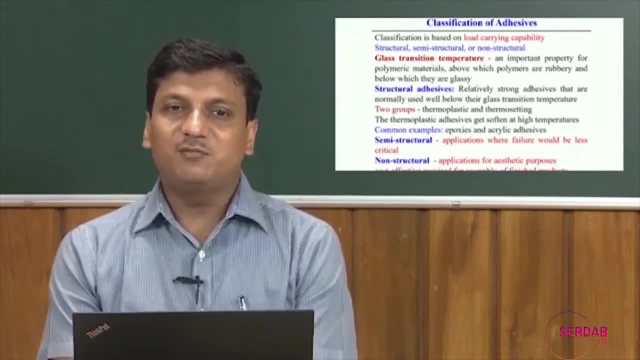 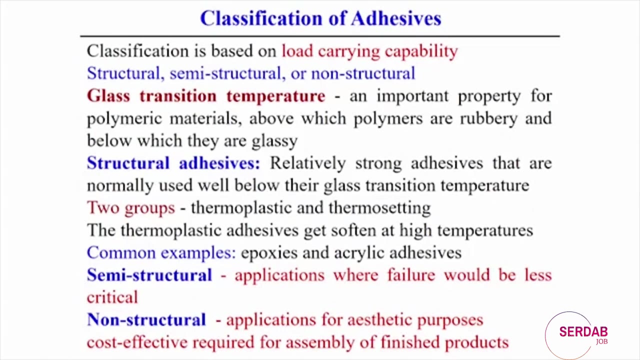 But thermosetting they becomes harder with respect to the temperature. So common examples of the structural adhesives are basically epoxies and this acrylic. these are the typical adhesives we use for the joining of the components. So if you look in the semi structural, in this case the application, where the failure would 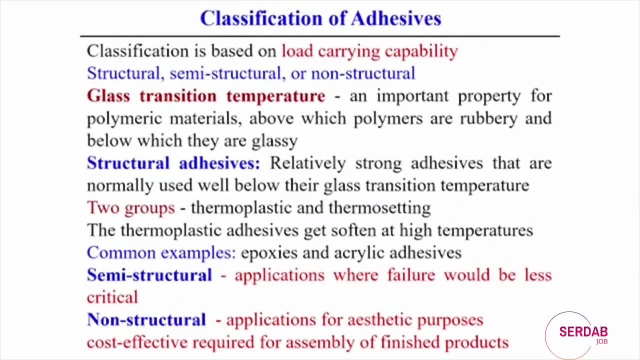 be the less Critical. so in this case the failure would be the less critical. we can use the semi structural adhesives or semi structural, joint and non structural. the strength is not important here, the non structural, here the application is done based on the aesthetic purposes. 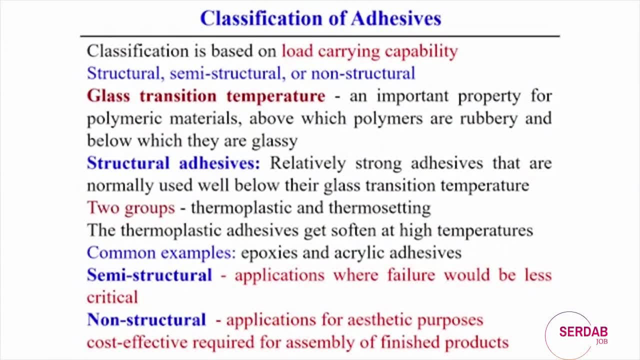 So these are the, if you look into that, three different types of the adhesives: the structural, semi structural and non structural adhesives. So these are the semistructural adhesives and, based on the load carrying capability, structural adhesive is the having the good load carrying capability. semi structural. 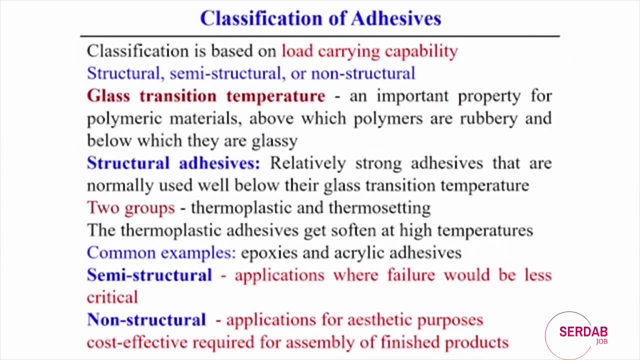 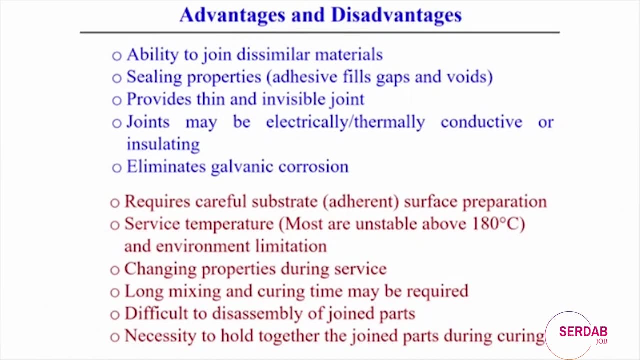 little less than that. and non structural they, when it is not the load. here the importance are given to the aesthetic purpose of this adhesives. So these adhesives are joined for. the adhesives are used for the joining of the components. 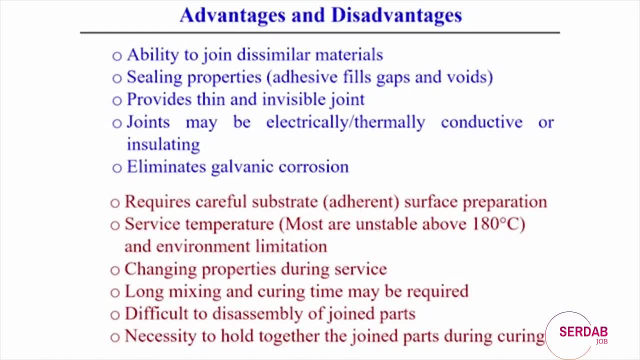 If you look into the overall, what are the advantages and the limitations of the adhesive joint? you can summarize like that: the ability to join disassembled materials. that is the one advantage for the adhesive bonding Definitely, which is the similar, typical to the other welding processes or like brazing and soldering. also, 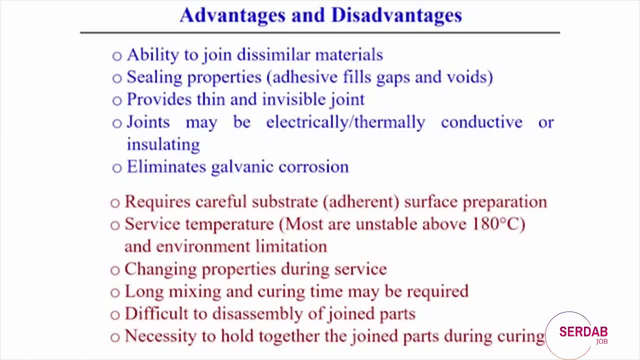 So sealing properties adhesives. it is having the good sealing properties using the adhesive because it generally try to fill the gaps and the voids And definitely adhesives sometime. most of the cases we use the very thin layer and invisible joint but good joint strength. 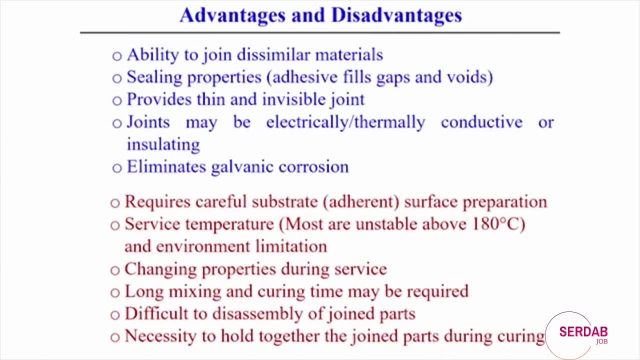 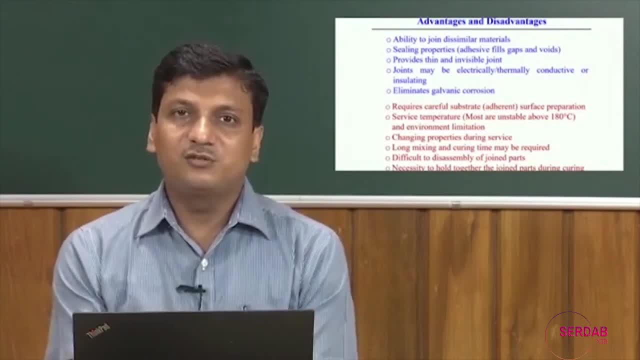 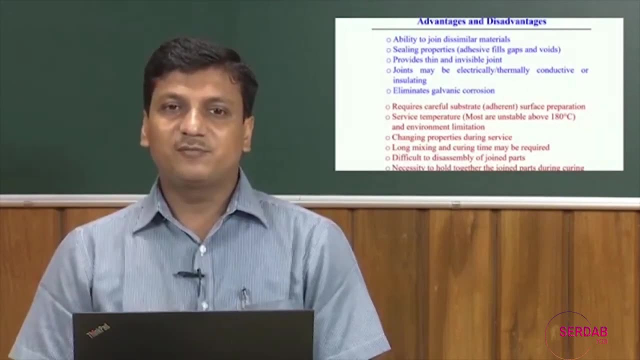 can be achieved, And the adhesives using some additive agent. the adhesives can be improved electrically or thermally conductive or insulating, whatever requirements are there, And that kind of flexibility is there also using this, using the adhesive joints between the components And of course, the adhesive joints is actually eliminates any of galvanic. 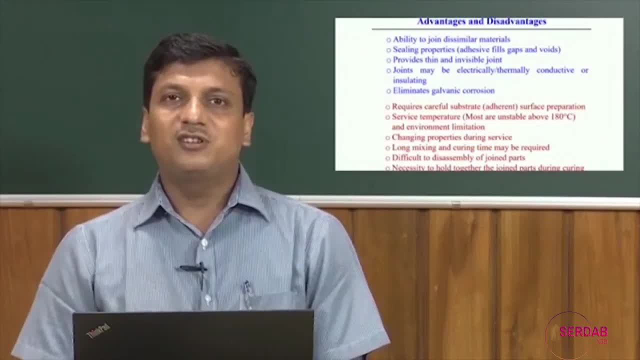 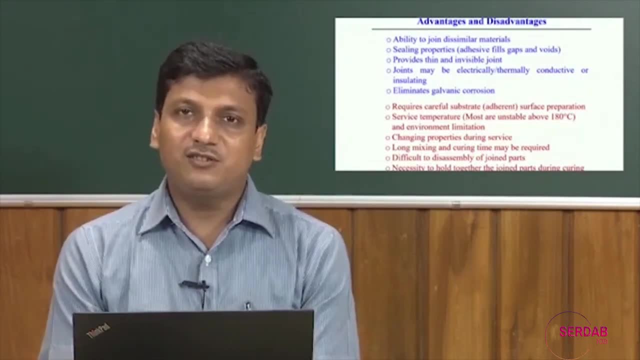 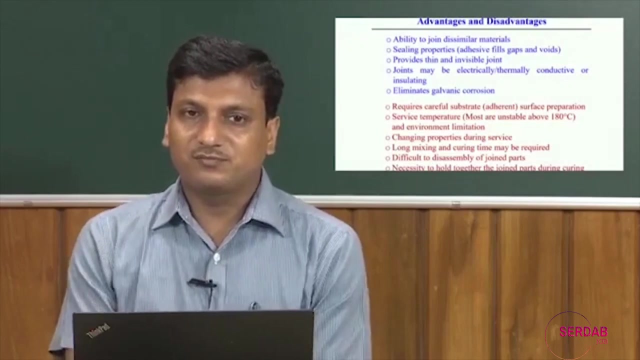 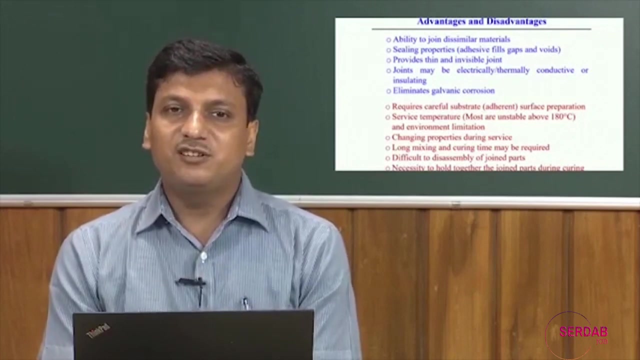 corrosion. So using these things, corrosion resistance can be improved using the. this adhesives on the, during the adhesive bonding or if you simply use the adhesive layer upon the any kind of components. But if we see the negative side, or may be disadvantage, of this adhesive bonding, the 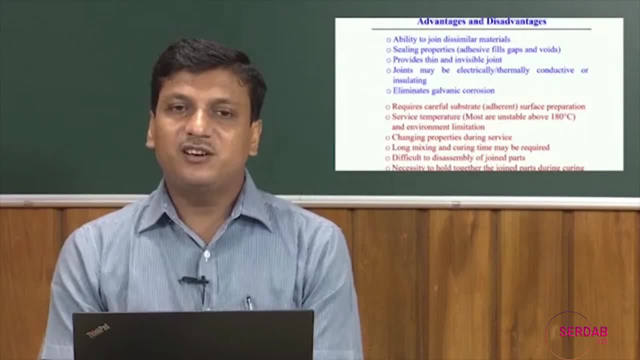 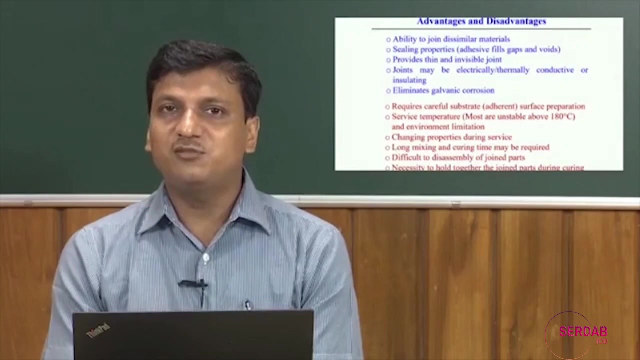 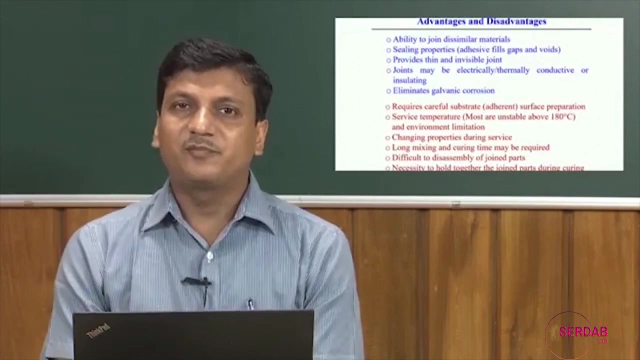 first is that requires careful substrate surface preparation. So surface preparation is one important factor. one is the cleanliness and the roughness. these two are the important parameters for the successful weld zone using the adhesive bonding Service. temperature and Milky lightning, and it is also here discussed, as the gi tenemos guys are coming back to. 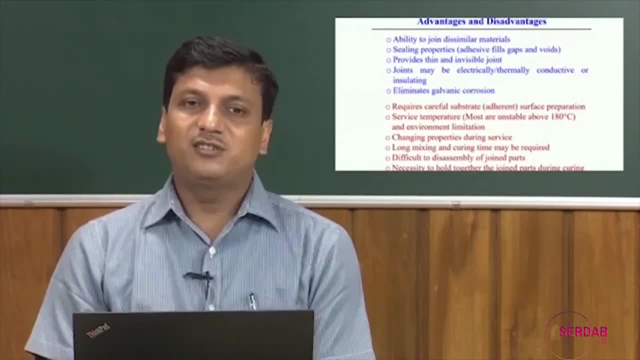 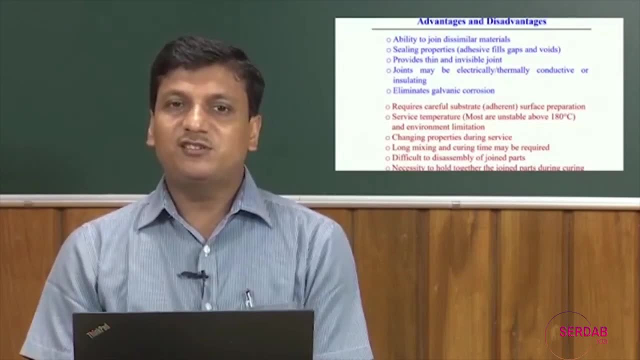 get to приб creepy limitation of this type of joining. It may change properties during the service. So that is another risk that if you cannot assess the changing properties during the service, 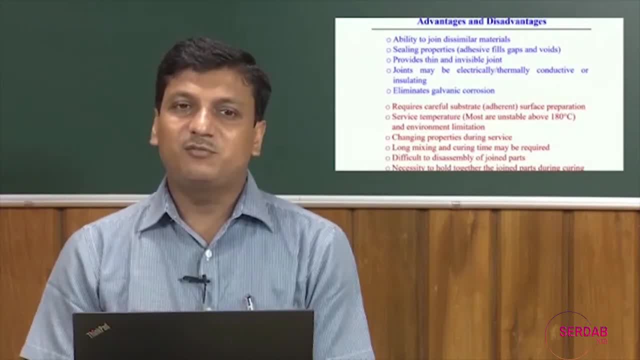 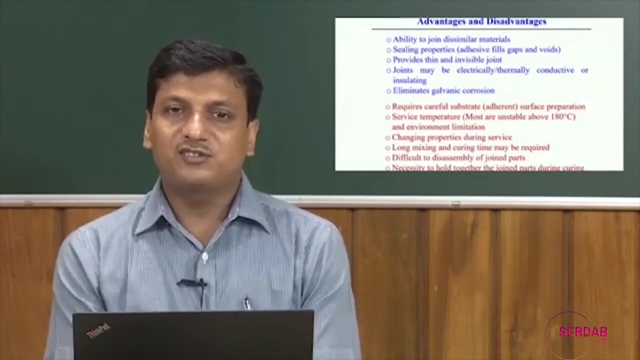 then probably it cannot be a very reliable join, reliable join process and the main in terms of the production of this process is the main disadvantage is that high curing time that makes the production time is very high for this adhesive bond. So this is another. 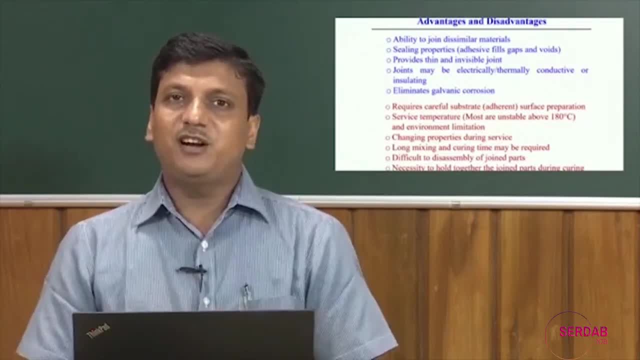 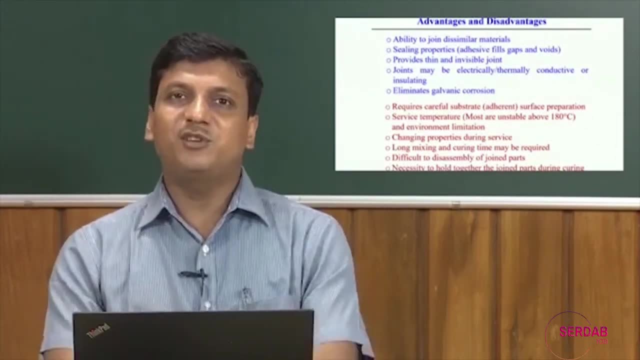 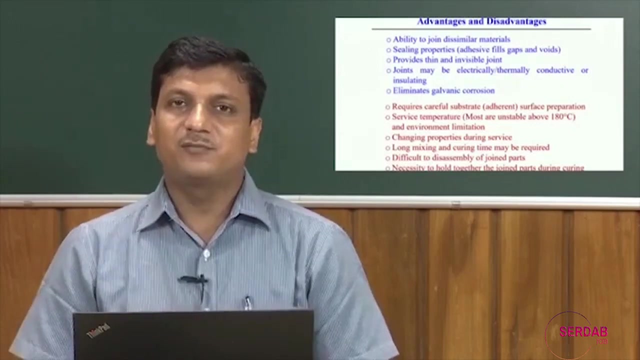 disadvantage and difficult to disassemble the joins. like soldering joint it is a simply by applying the heat we can easily disassemble of the joint. But once the adhesive bond has occurs between these two components then it is difficult to disassemble again.